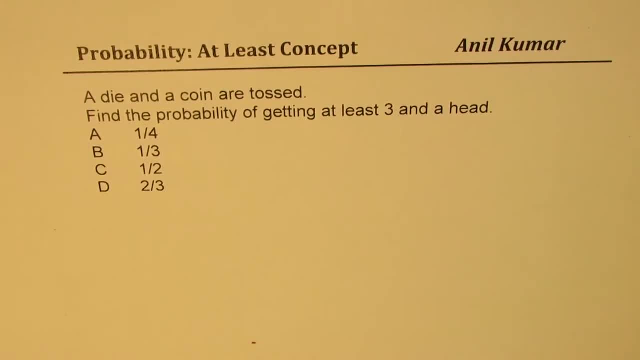 Hi, I'm Anil Kumar. Welcome to my series on multiple choice questions, And these questions are going to help you in many competitive exams. The example here is: a die and a coin are tossed. Find the probability of getting at least three and a head. So when we are saying a die, we are talking about a fair dice which is kind of like this: 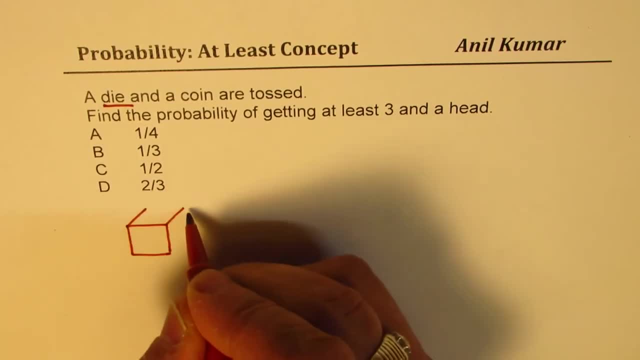 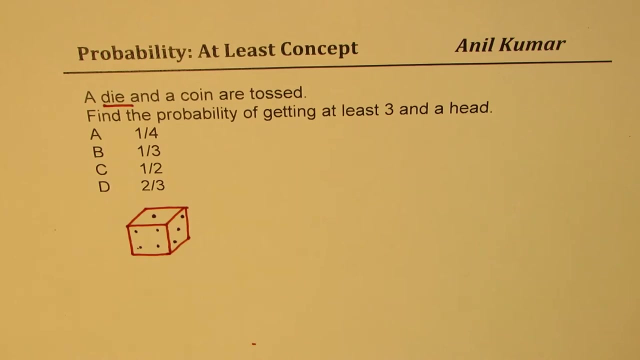 Correct. So we have a dice here. Let's say Okay, so they are tossed. The probability of getting at least three and a head, That is what we're looking for. So when a dice is cost, tossed we could get numbers from one to six, and for a coin we could get head or a tail. 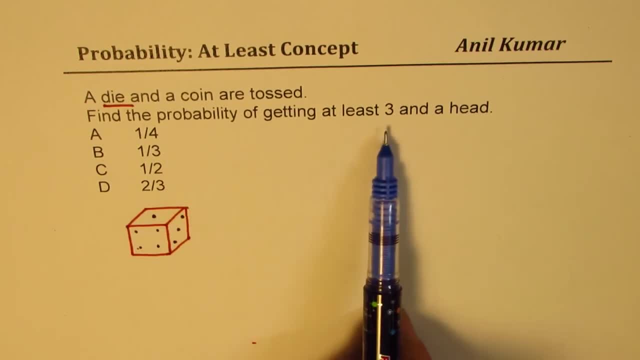 so you need to find the probability of getting at least three and a head. so i like you to pause the video, answer the question and then look into my suggestions. correct now, what do you mean by at least three? that really means that we are looking for numbers which are three, four, five and six. 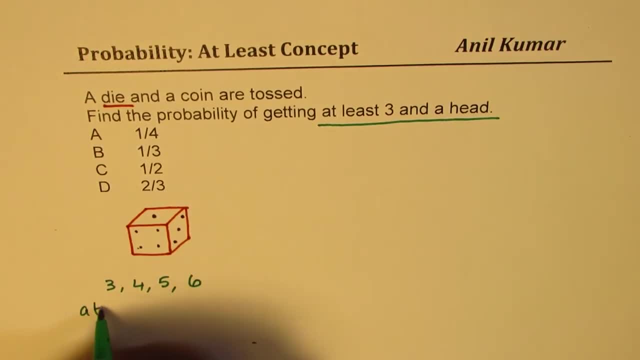 that is at least three. right? this is what we mean when we say at least three. perfect now. i think it becomes absolutely clear and you can easily find the solution: perfect now. there are many ways to go about. let us make a tree diagram to get to the solution. 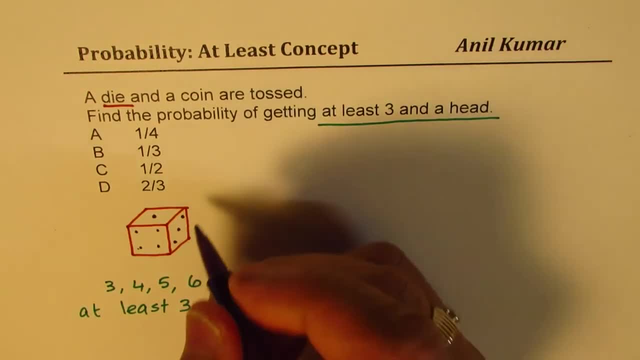 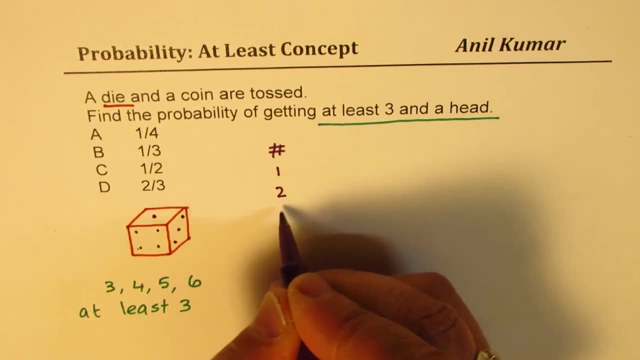 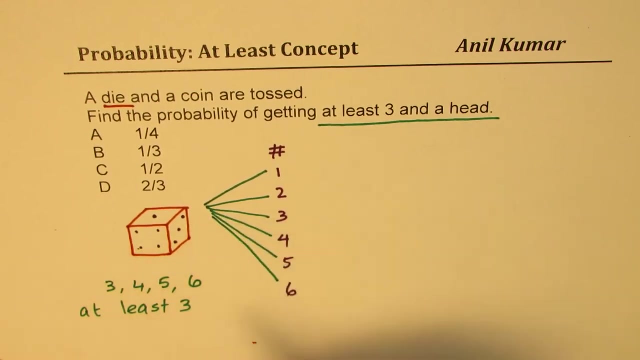 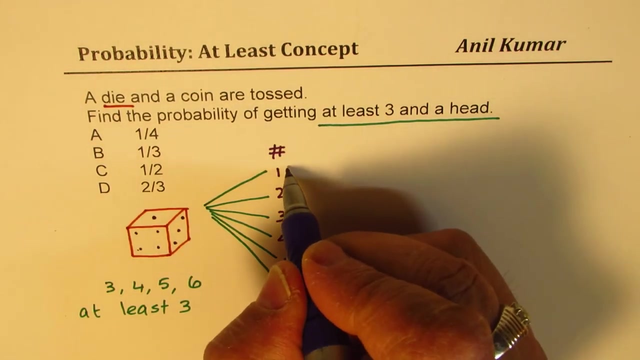 so so. so the possibility for the numbers is what we could get: one, two, three, four, five or six. so these are the possible numbers which you could get from the given dice, and for each combination you could either get a head or a tail right. so, for example, 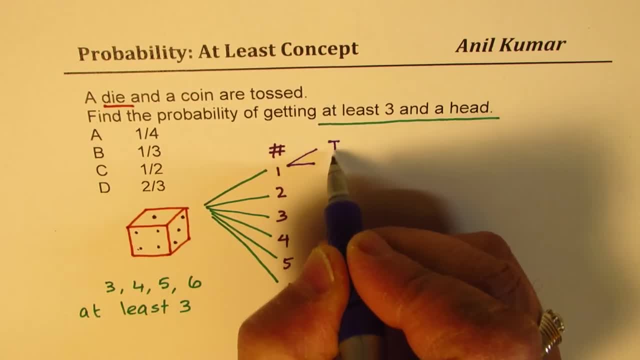 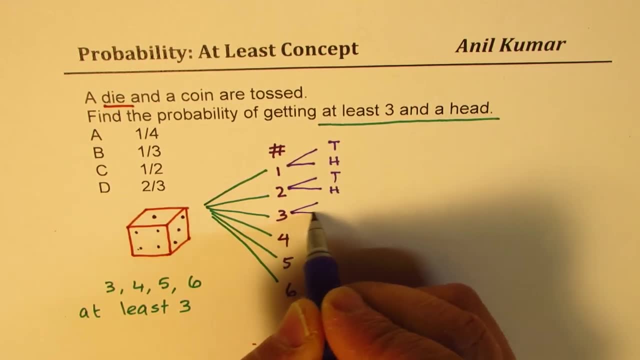 you could get a head or a tail right. so, for example, if you get a head or a tail right, so for example, For each combination you have two possibilities: You could get a tail or a head right. So for each we have two: we could get a tail or a head. 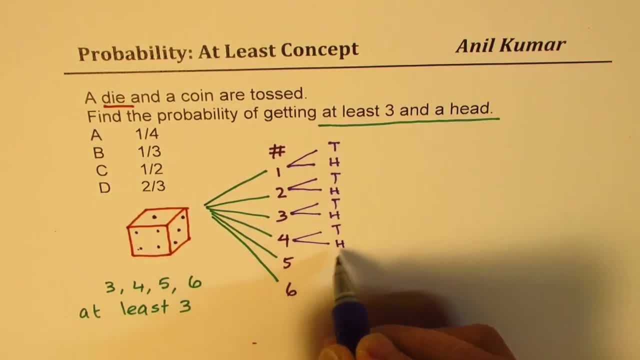 So I hope that is absolutely clear. Now I'm making these three diagrams so that you could visually see what is happening and how to get the result In a competitive exam. however, you're not going to do all this correct, But this will help you to visualize and get a quick answer. 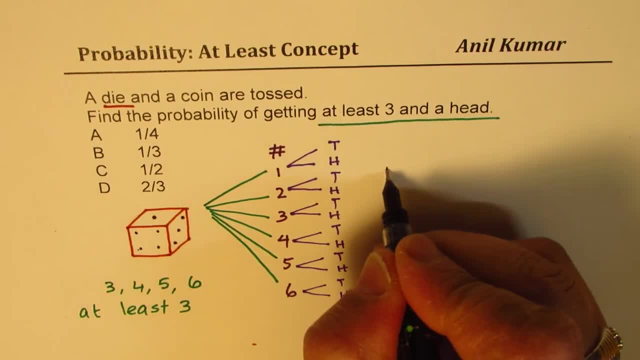 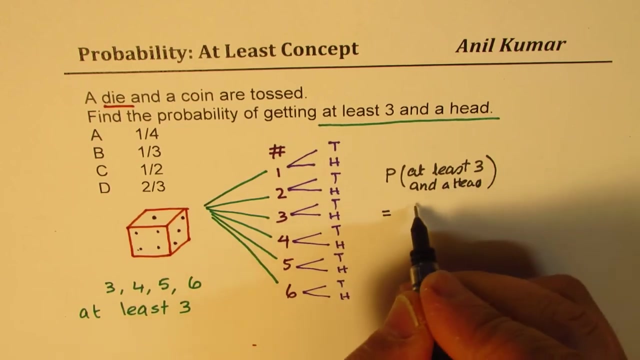 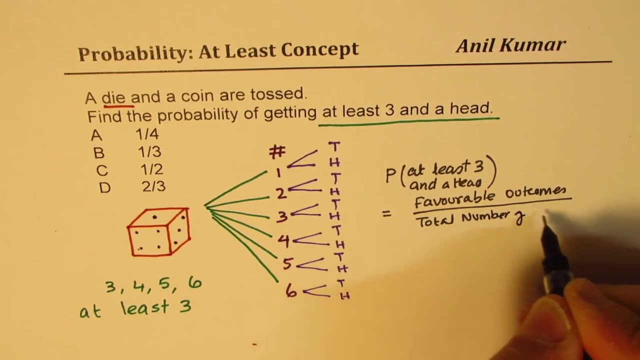 Now, when we say probability, we're talking about we want at least three and a head, So the probability is always favorable. outcomes over probability. Total outcomes correct. Now, total number here is six times two, So we could write this total very easily here. 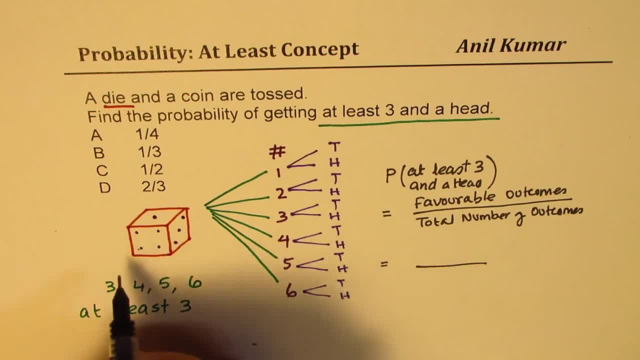 So initially, as far as dice is concerned, total outcomes are from one to six, correct? So here we have six possibilities and here we have two. So when you multiply six and two, you get your total number of outcomes, which is 12.. 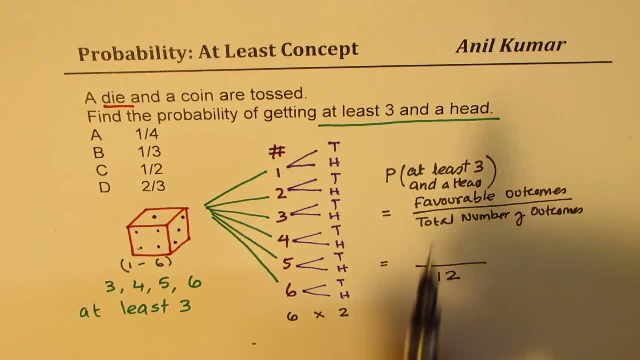 Okay, Perfect. Now we're looking for at least three. That means for the dice the number should be three, four, five or six. That means these are four, right, And for each four we have only one possibility of getting head right. 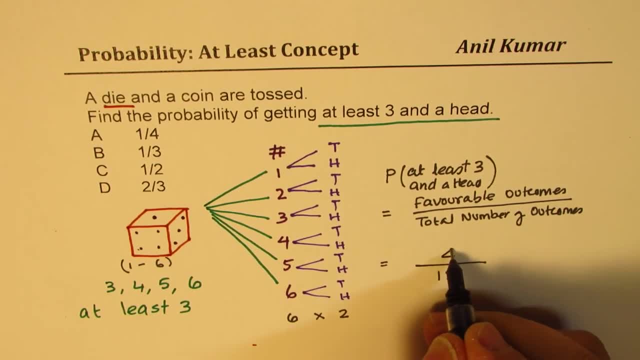 So we get here four times one, which is four on the top, correct. Now, when you make a tree diagram, how does it help? It helps you to visualize. So that's the whole idea, So we could actually visualize from here. 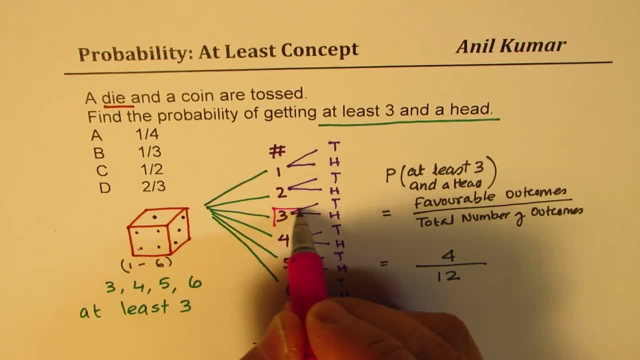 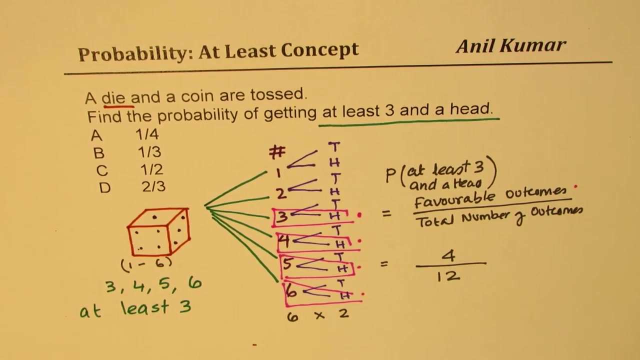 And see what our outcomes are. So tail, I mean three and head, four and head, five and head and six and head. So these are the four favorable outcomes, correct? So we get four over 12 as our answer. 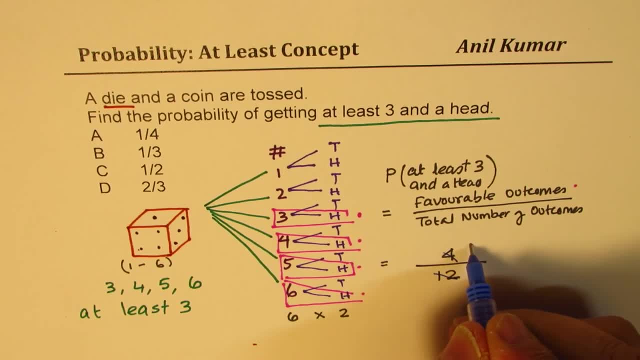 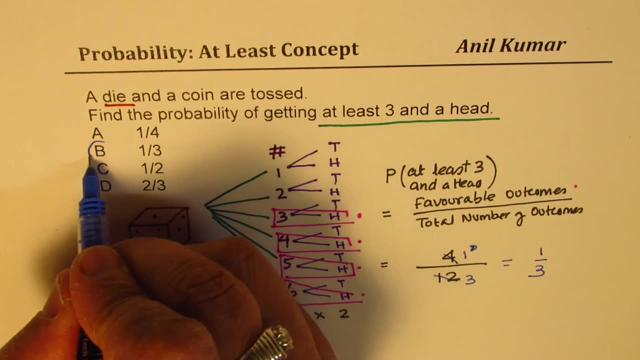 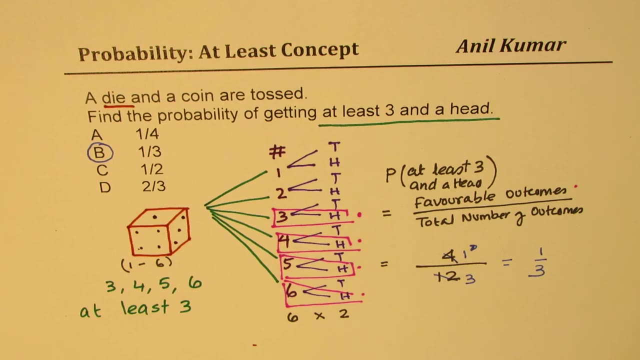 So when you simplify this, both could be divided by four, So you get one, and here you get three. So the answer is one over three. Option B is the right option, Perfect. So I hope that is absolutely clear. Now, if you get this question in multiple choice test, then what you need to do is straightaway.